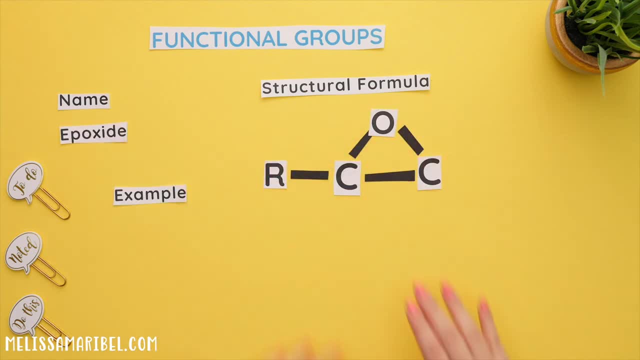 from the other. An epoxide has a triangular shape, with the oxygen being at the top of this triangle-shaped carbon chain. A ketone has a carbon that is double bonded to oxygen and that carbon is attached to two R groups. This is a double bonded carbon chain and 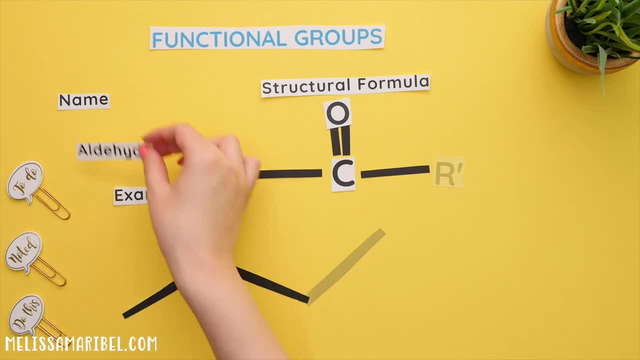 an aldehyde is very similar to a ketone. The only difference is that it has a hydrogen instead of two R groups. A trick to remember this is that aldehyde has an H in it. A carboxylic acid still has the same carbon, double bonded to oxygen, but 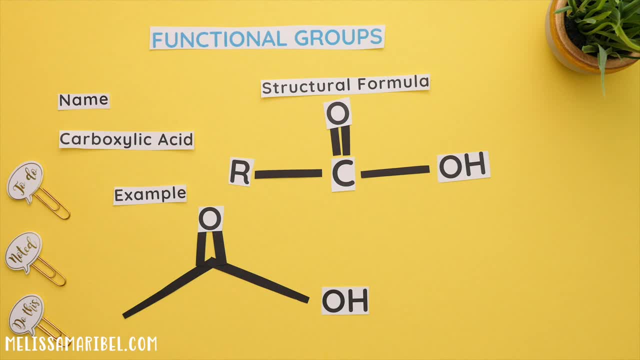 now there is an OH instead of an R group or hydrogen. An ester has a similar structure. An acetylcholine has a carbon double bonded to oxygen, but now there is an OH instead of an R group or hydrogen. An ester has a similar structure. 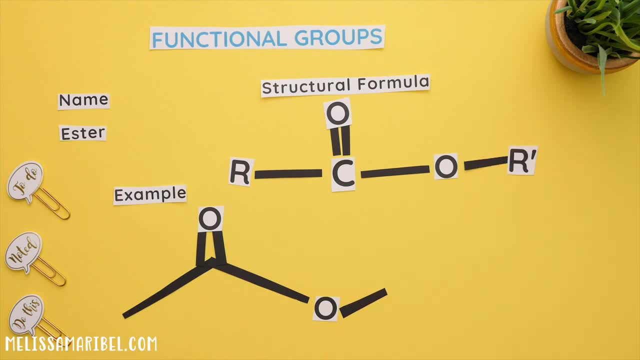 It just has an R group attached to the oxygen instead of a hydrogen. An amide now has a nitrogen attached to the carbon that is double bonded to the oxygen. An amine still has nitrogen but it does not have a carbon double bonded to an oxygen. To remember the difference between: 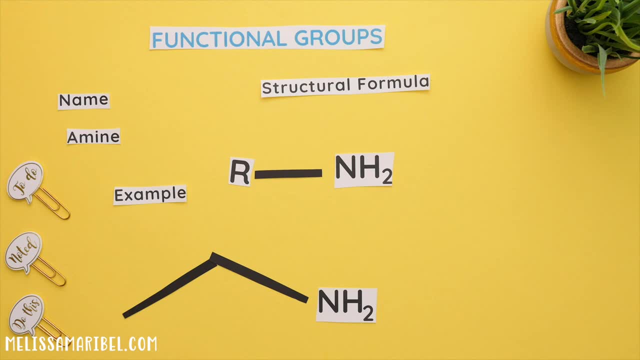 an amide and an amine. it's hidden in the name. An amine has the minimum amount of atoms, so it's the one without the H. So what could happen to the oxygen? An amide has the minimum amount of atoms, so it's the one without the oxygen. 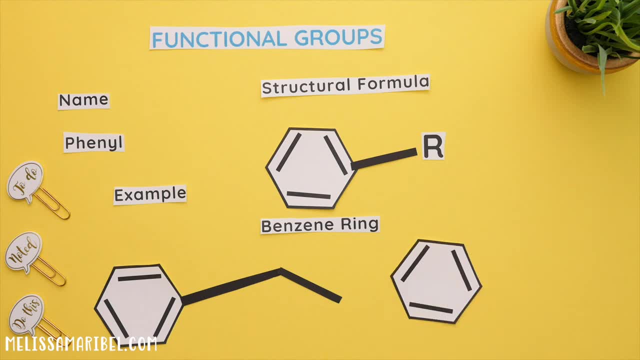 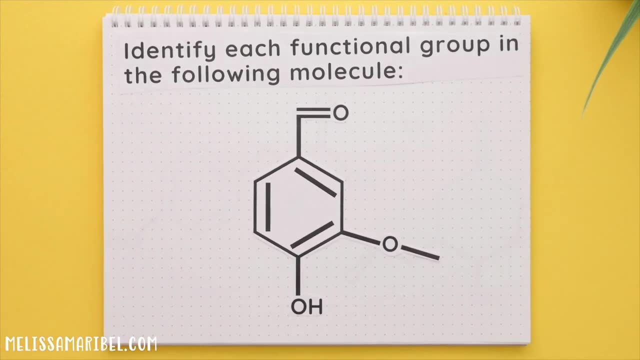 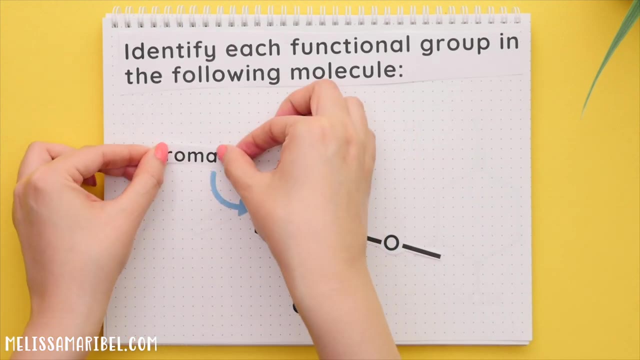 And this is a phenyl group where a benzene ring is attached to an R group. Another functional group name is aromatic. This describes a benzene ring. Okay, here is a potential quiz or test question. We are asked to identify each functional. 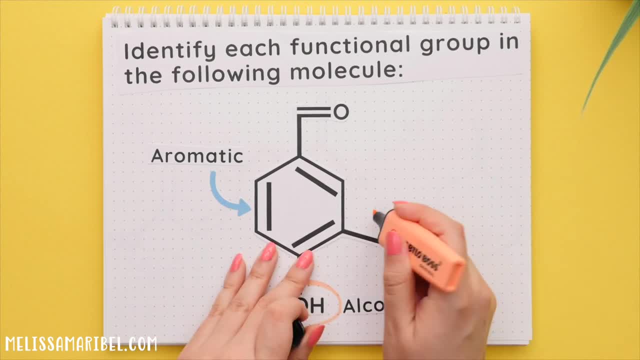 group in the following molecule. We have a benzene ring which is aromatic. This OH tells us it's an alcohol. Here we have two R groups and an oxygen. We have a benzene ring which is aromatic. This OH tells us it's an alcohol. 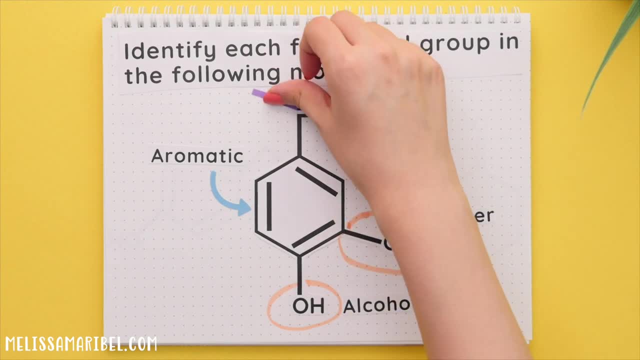 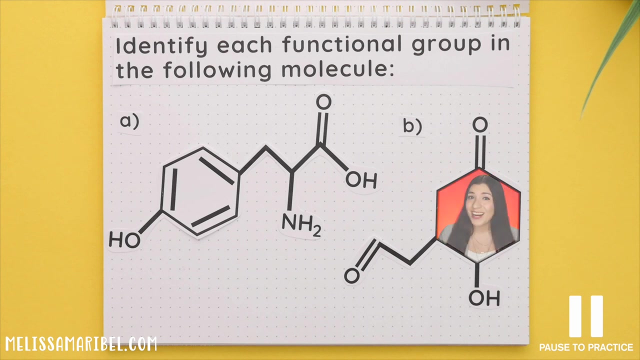 in the center, which is an ether, And on top note, there is actually a hydrogen here, making this an aldehyde. Okay, try these two on your own, and then I'll walk you through all of the answers, plus I'll let you know what common mistakes to look out for.